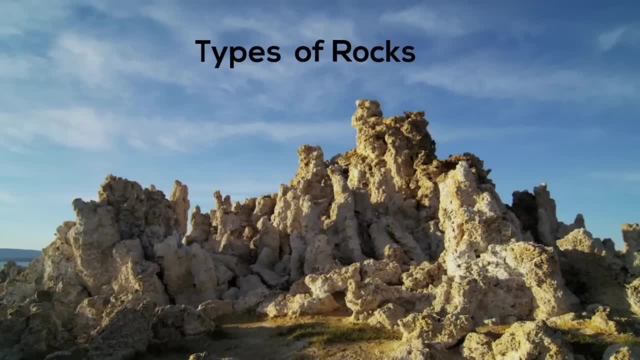 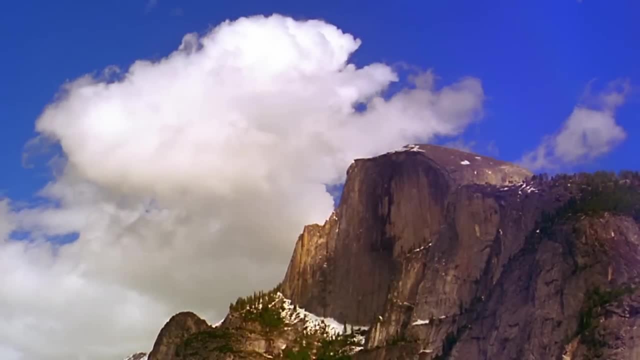 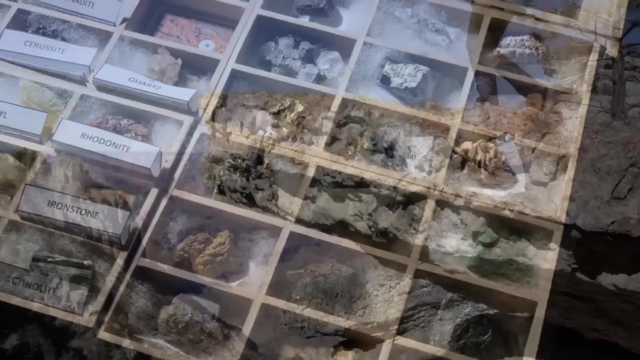 Welcome to MooMooMath and Science. In this video, let's take a look at the different types of rocks. Rocks are all around us. They make up this famous formation called half dome or the smaller rock formation. They can be small or seen in these canyons. A rock is a solid, naturally occurring. 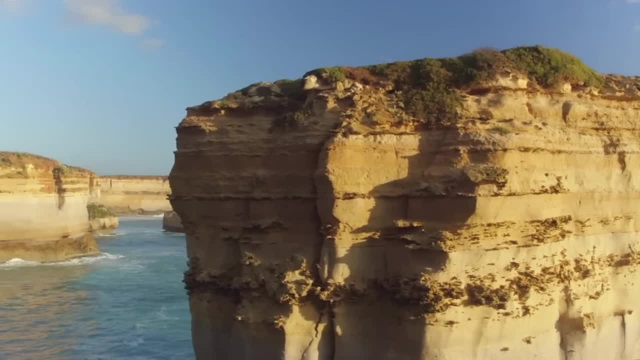 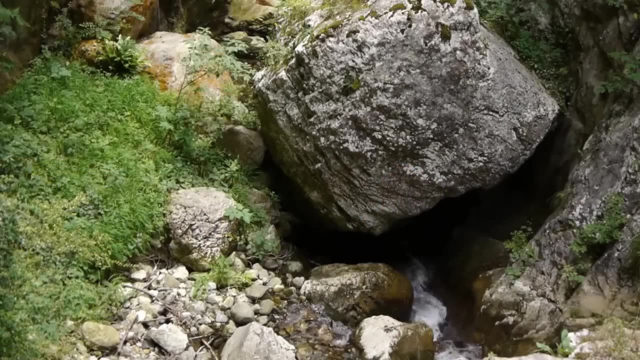 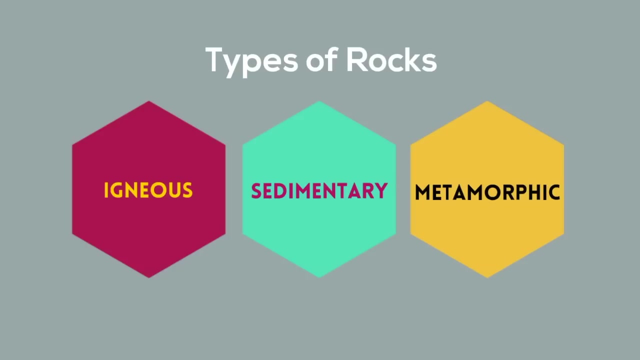 rock and is made up of minerals or mineral like matter, like shells. Rocks can be divided into three basic types, depending on how they are formed. These types are igneous, sedimentary and metamorphic. Let's take a look at these different types of rocks. 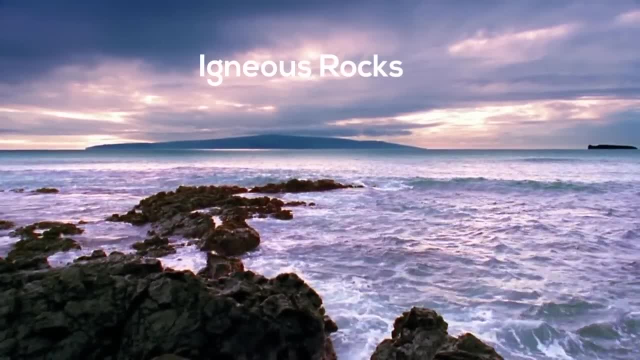 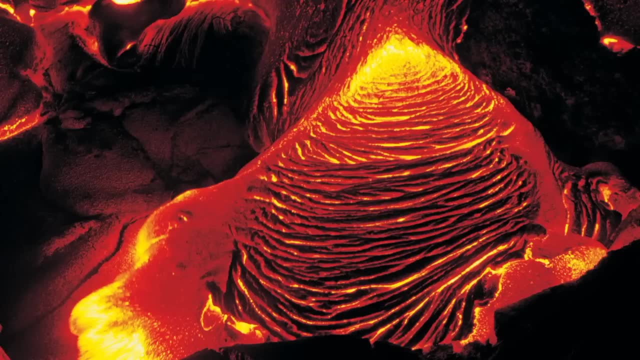 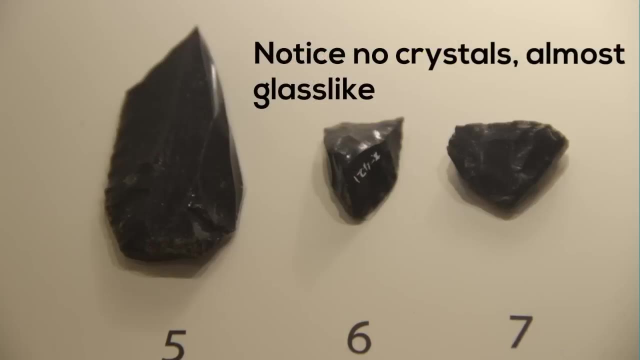 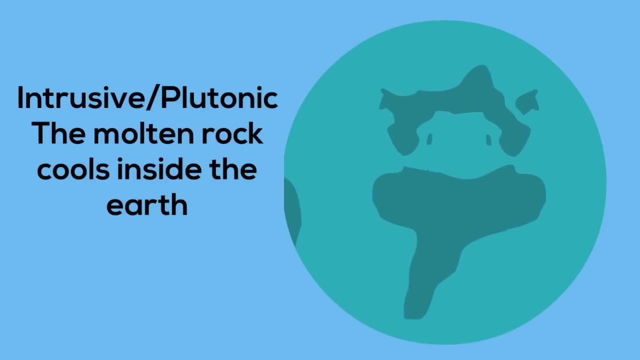 Igneous rocks are formed when magma or molten rock cools. This magma can either flow to the surface of the earth and cool quickly- and these rocks are called extrusive or volcanic igneous rocks, and they generally have very small crystals- Or they can cool inside the earth, and these are called intrusive or 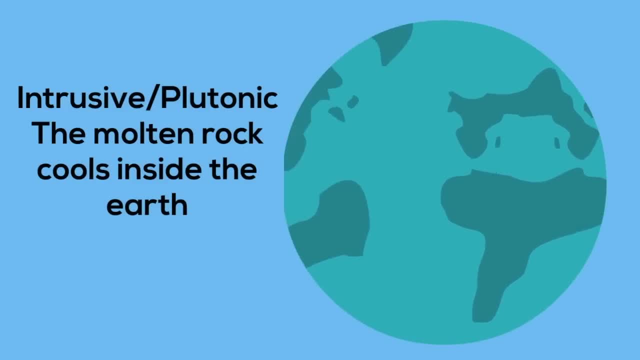 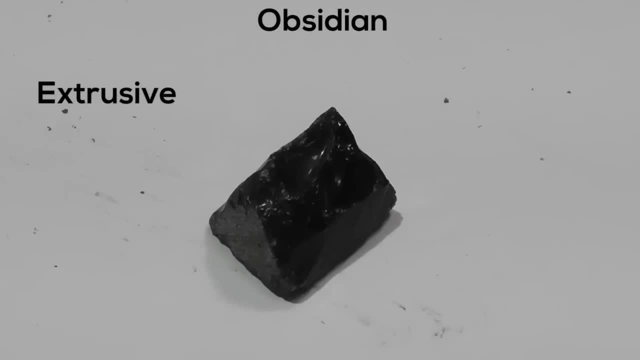 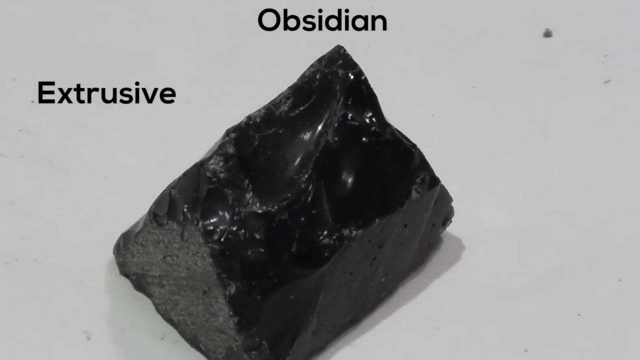 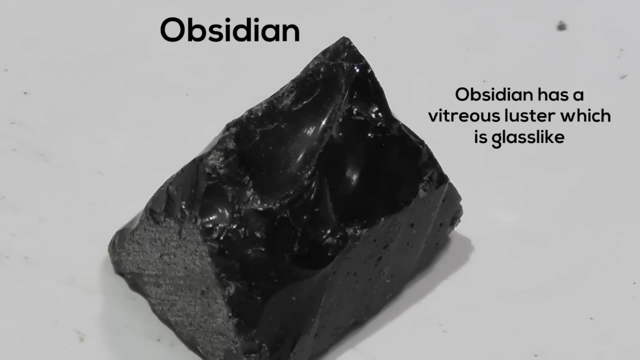 plutonic rocks, and they generally have larger crystals than the extrusive, igneous rocks. So up, first let's take a look at obsidian. Obsidian is an igneous, extrusive or volcanic rock. It is made up of quartz, alkali and field spar. It looks like glass and has a hardness. 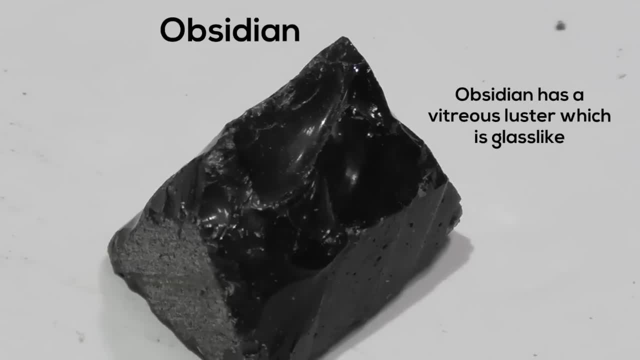 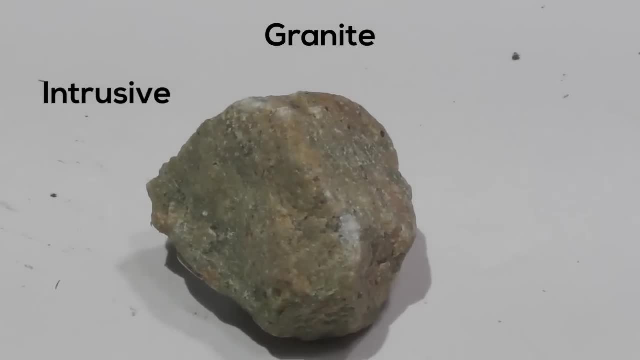 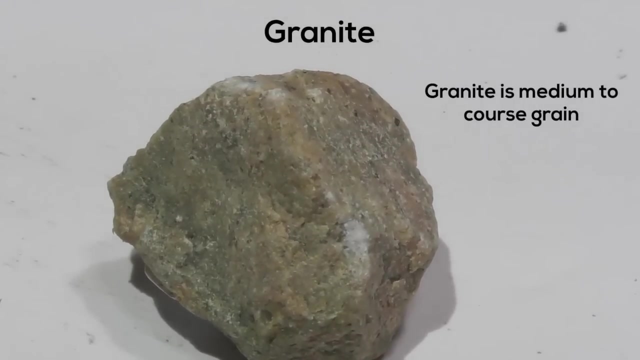 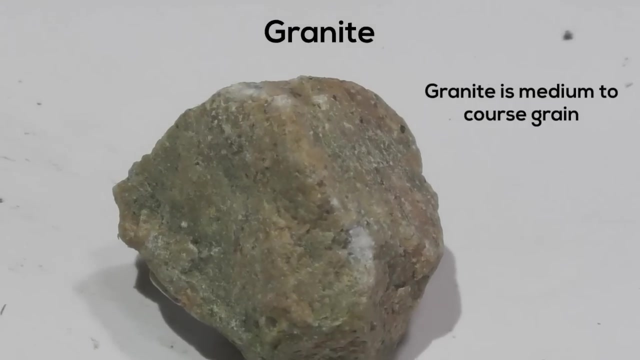 between 6 and 7.. So there is obsidian. Next we have granite. Granite is an igneous, intrusive or plutonic rock. It is made up of field spar, quartz and mica. It has medium to coarse grain crystals and a hardness between 5 and 5.5.. 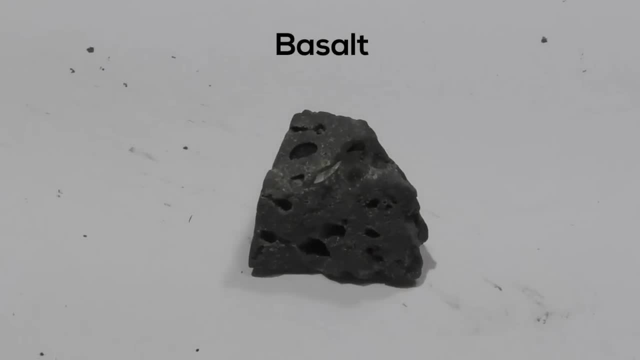 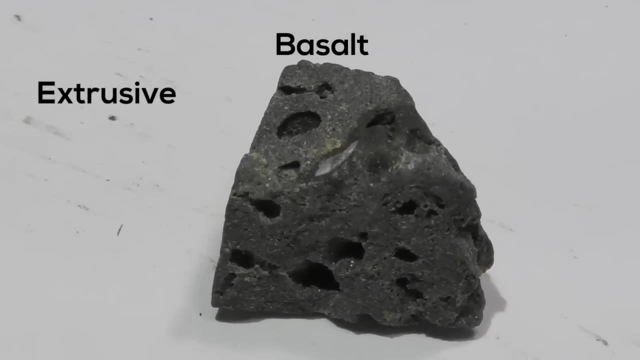 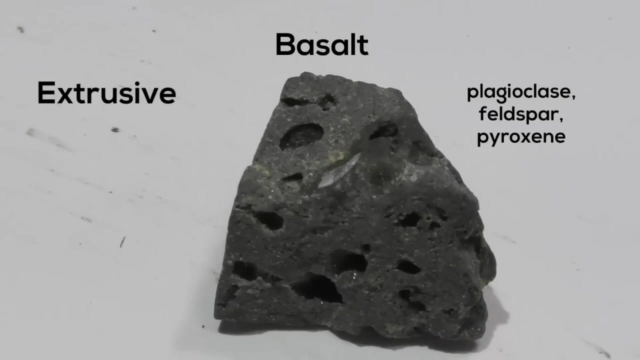 Next is basalt. It is an igneous extrusive rock. It is made up of plagioclase, field spar and pyroxene. It is dark and dense and is very fine grained. Next we have basalt. It is an igneous extrusive rock. It is made up of plagioclase, field spar and pyroxene. 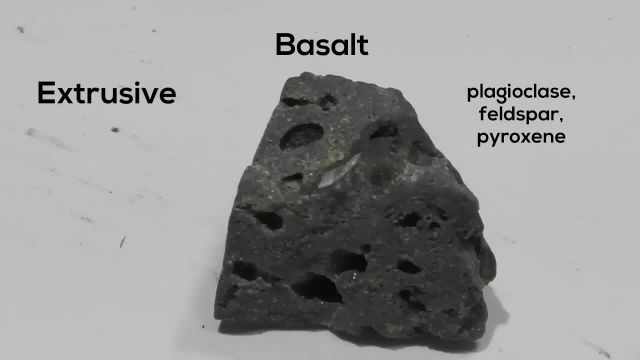 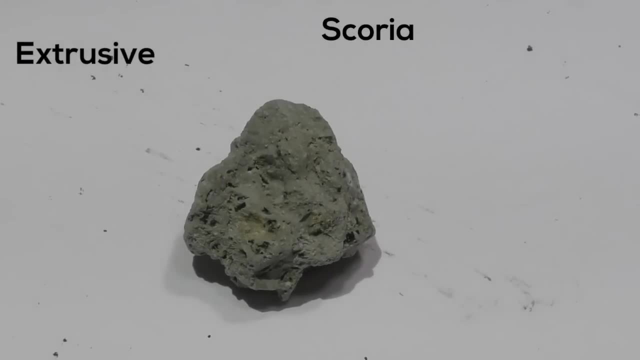 It is dark and dense and is very fine grained. It has a hardness between 5 and 6.. So there is basalt. Next we have scoria. It is an igneous volcanic rock. It is made up of field spar. 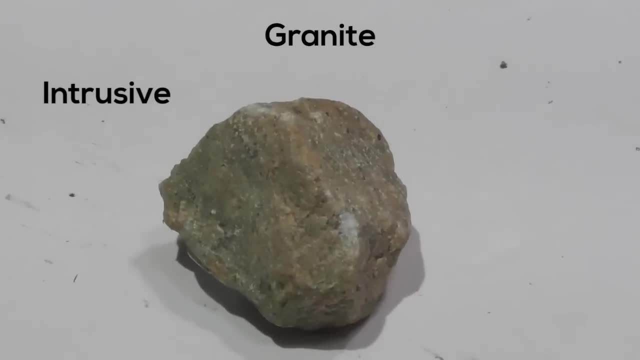 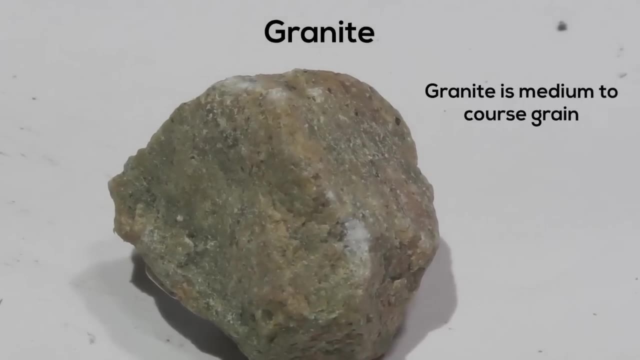 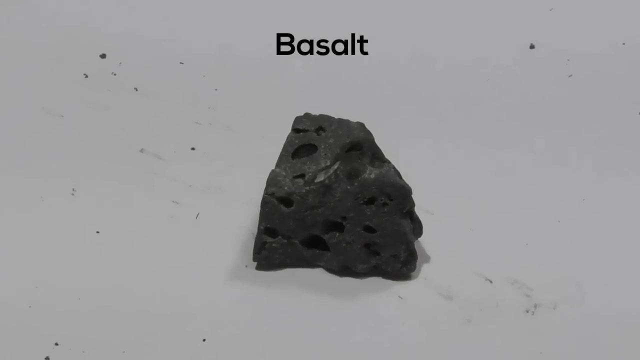 Next we have granite Granite is an igneous, intrusive or plutonic rock. It is made up of field spar, quartz and mica. It has medium to coarse green crystals and a hardness between 5 and 5.5.. Next is basalt. It is an igneous, extrusive rock. It is made up of plagioclase field. 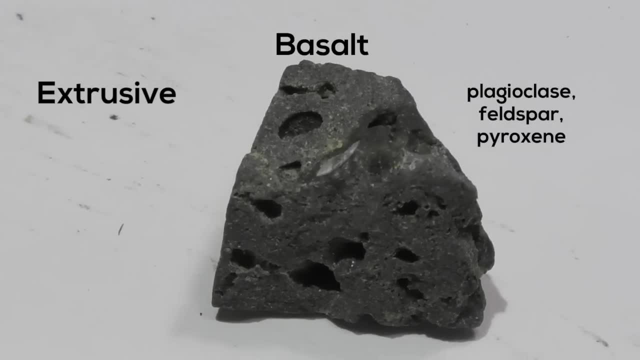 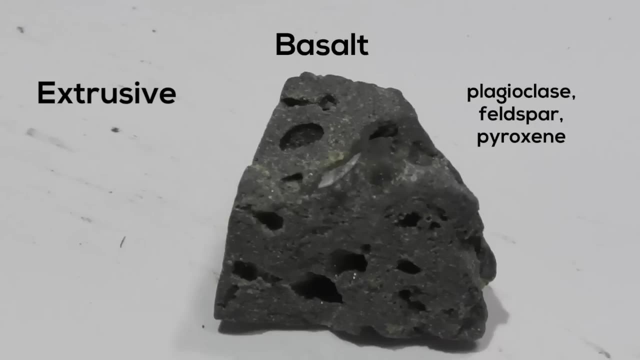 spar and pyroxene. It is dark and has a high concentration of calcium. It is also made up of basalt. It is dark and dense and is very fine grained and has a hardness between 5 and 6. So there is basalt. 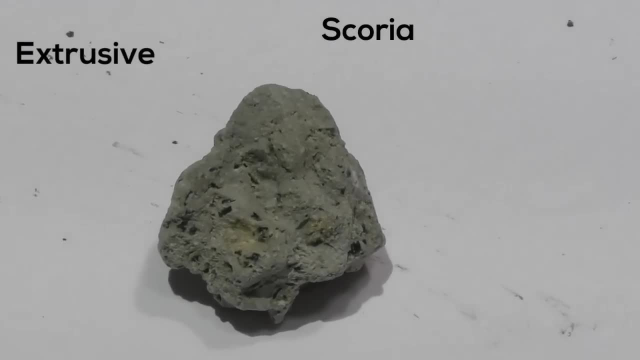 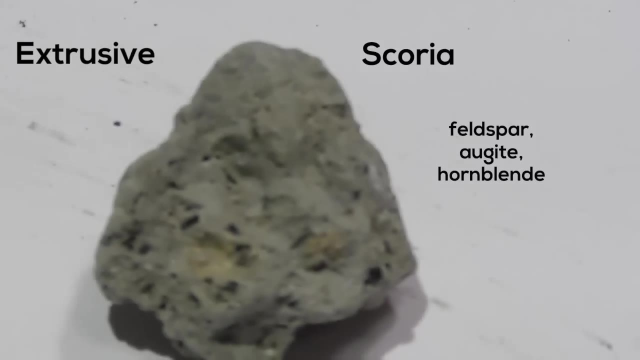 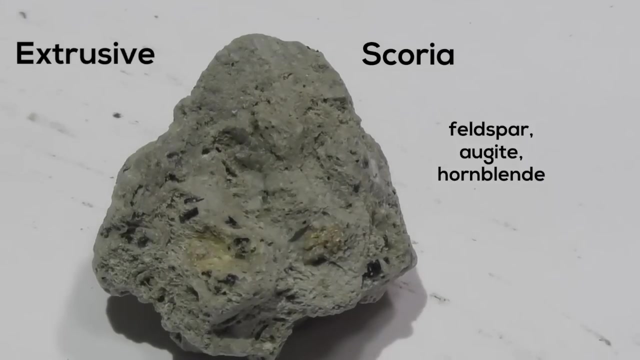 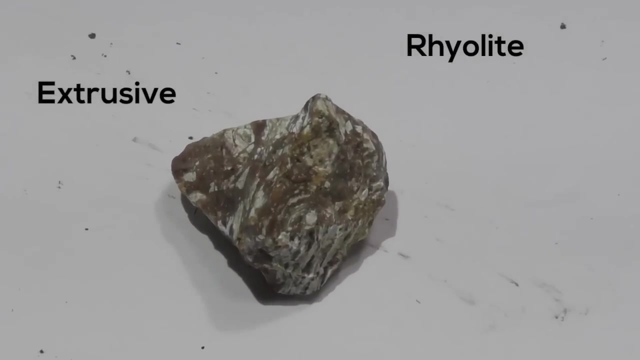 Next we have scoria. It is an igneous volcanic rock. It is made up of field spar, algite and also hornblende. It is basalt with cavities filled with other minerals. It is made up of gradation of citric acid, polyethylene and lanine oxide. It is a very fine grained rock. 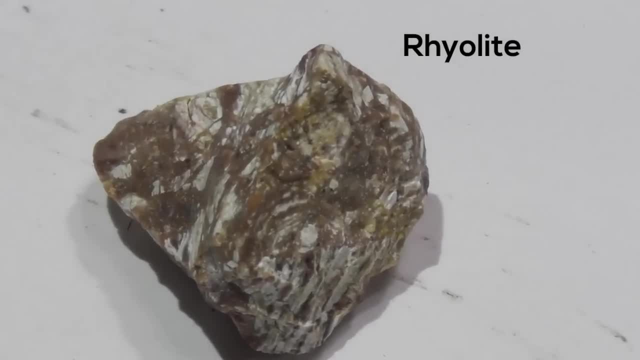 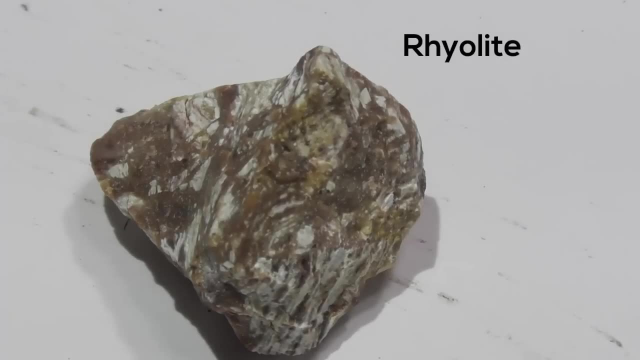 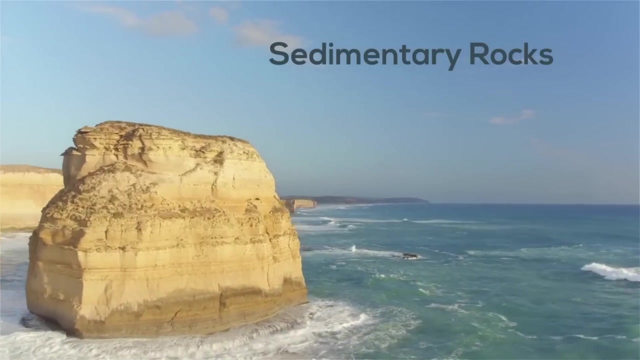 Finally, we have rhyolite. It is an igneous extrusive rock. It is made up of field spar, quartz and mica. It has a very fine grained texture and often it has a porous texture And it can float in water. 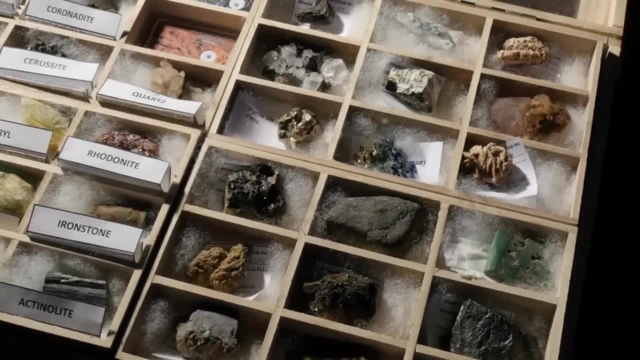 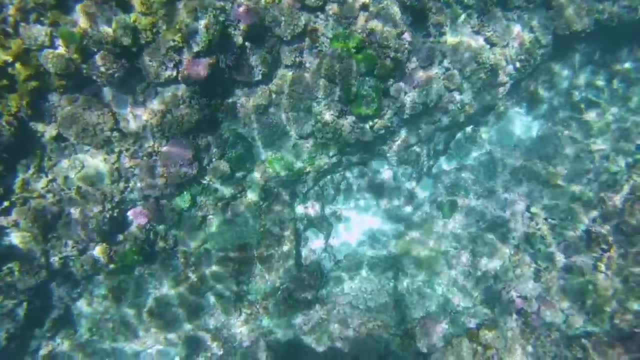 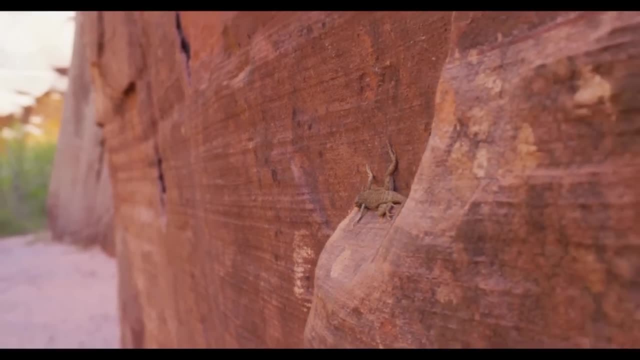 So there we go. 5 igneous rocks organisms. They form from deposits that accumulate on the earth's surface or under the ocean. These particles that form a sedimentary rock are called sediment and may be composed of minerals or once living matter called organic matter. Sedimentary rocks can be divided into several. 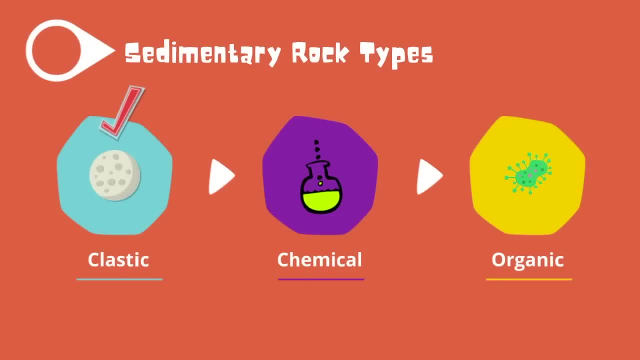 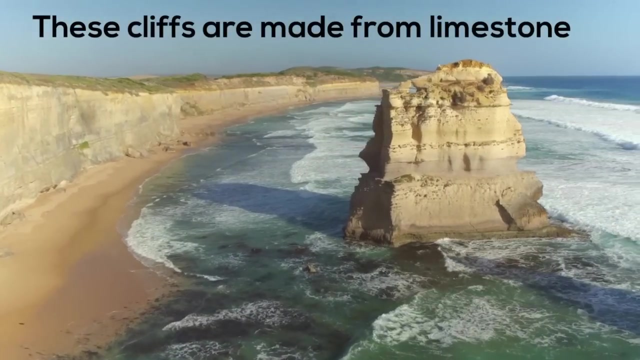 groups. Some common groups include clastic sedimentary rocks, which form from fragments of pre-existing rocks. Chemical sedimentary rocks, which form by precipitation of minerals from water- Precipitation is when dissolved minerals come out of water- And organic sedimentary rocks, such as coal and limestone, which form from the accumulation of plant and animal debris. 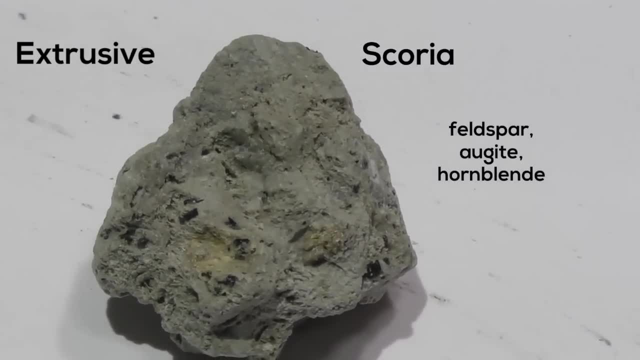 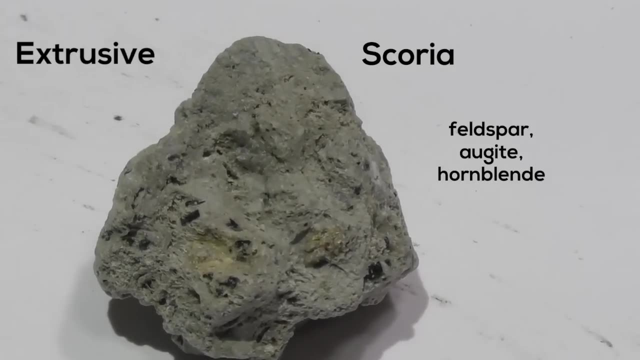 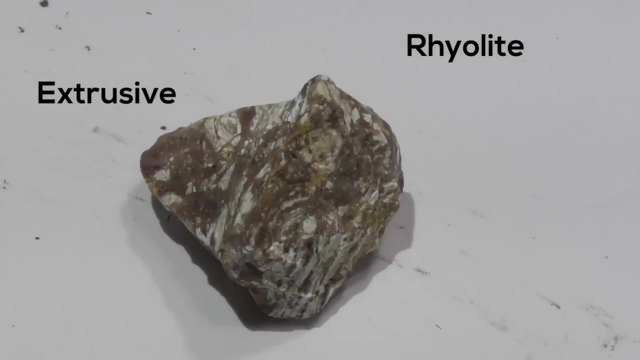 algite and hornblende. It is basalt with cavities filled with other minerals. And finally we have rhyolite. It is an igneous extrusive rock. It is made up of field spar, quartz and mica. 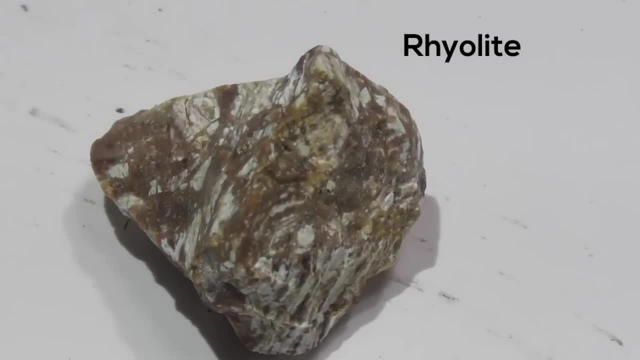 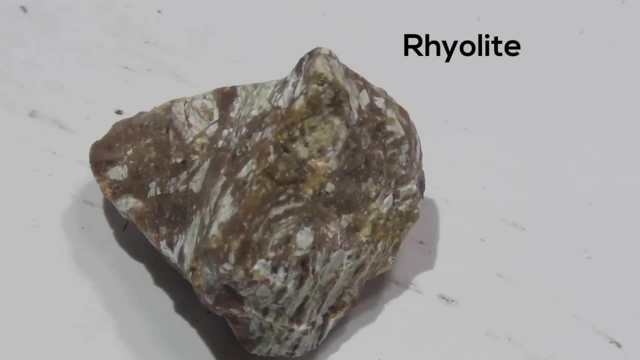 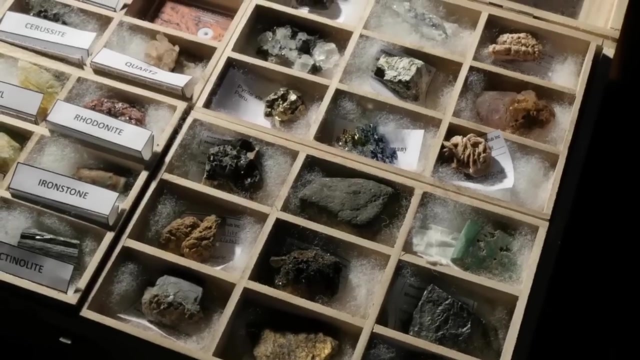 It has a very fine texture. It has a porous texture. It can float in water. So there we go, Five igneous rocks. Sedimentary rocks are formed from pre-existing rocks or pieces of once living organisms. They form from deposits that accumulate on the earth's surface. They form from deposits that 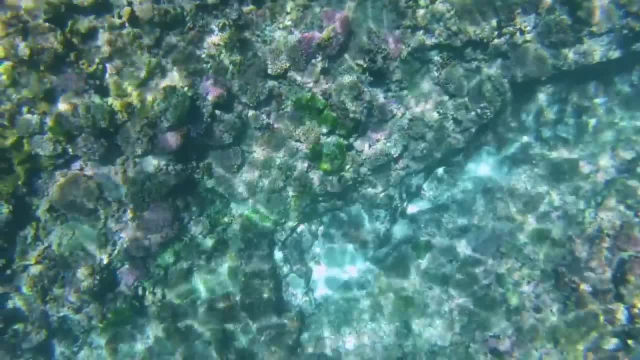 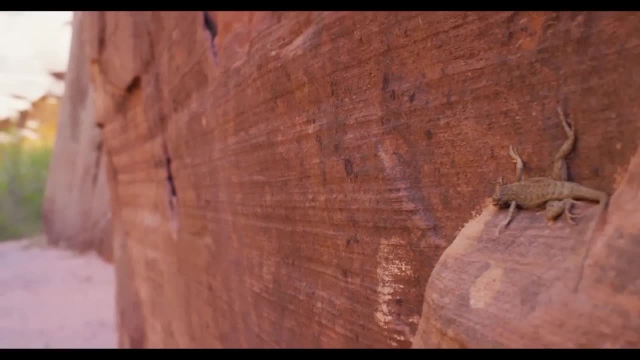 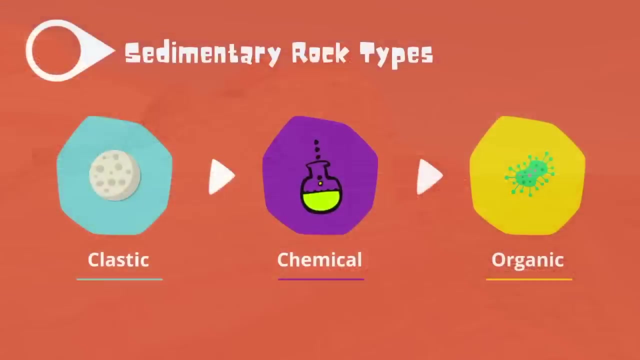 accumulate on the earth's surface or under the ocean. These particles that form a sedimentary rock are called sediment and may be composed of minerals or once living matter called organic matter. Sedimentary rocks can be divided into several groups. Some common groups include clastic sedimentary rocks, which form from fragments of pre-existing rocks. 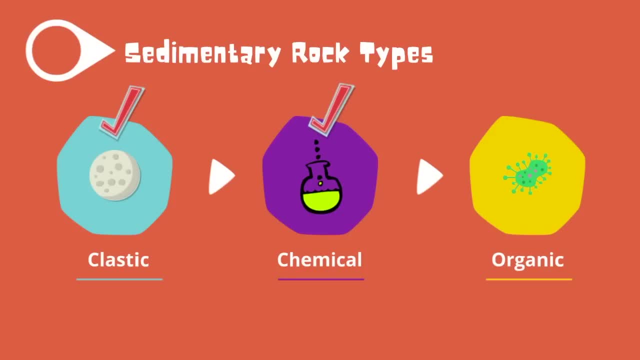 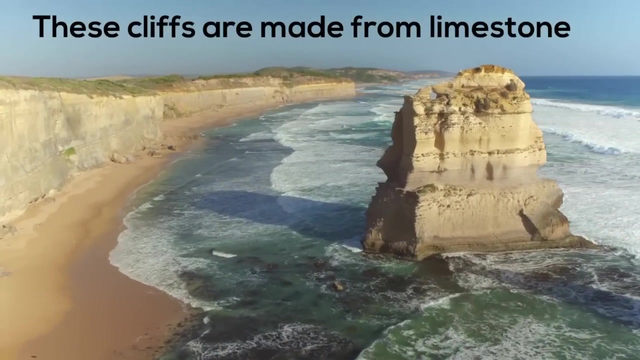 chemical sedimentary rocks, which form by precipitation of minerals from water- precipitation is when dissolved minerals come out of water- and organic sedimentary rocks, such as coal and limestone, which form from the accumulation of plant and animal debris. Clastic sedimentary rocks are subdivided according to the dominant particle size. 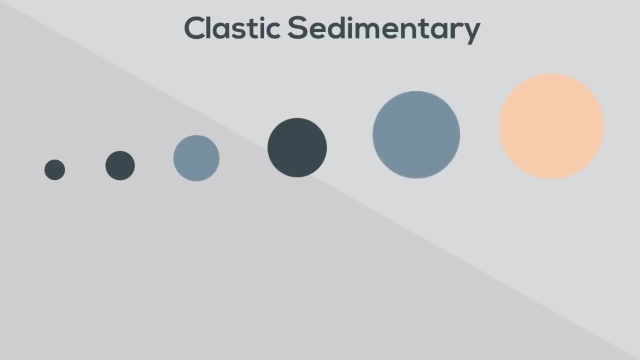 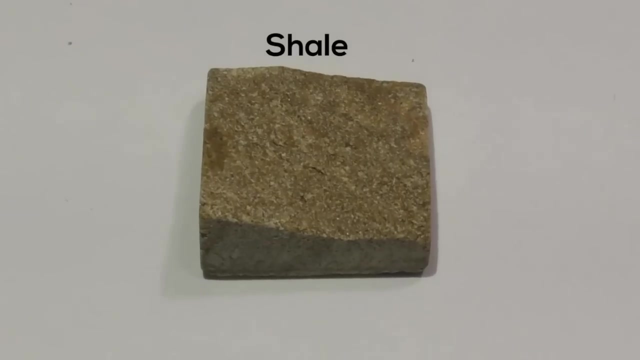 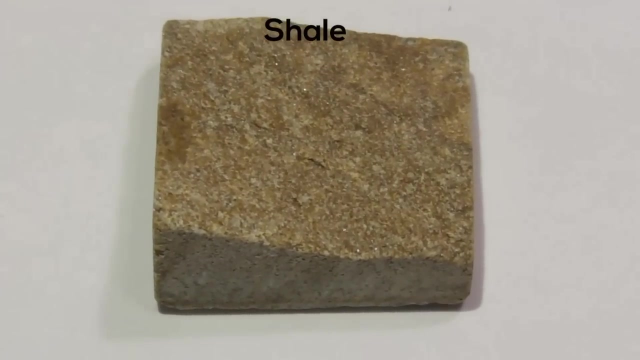 These particle sizes are ranked from smallest to largest: Clay is the smallest, then silt, sand, gravel, pebble and boulder. Shell is a fine-grain clastic sedimentary rock composed of mud. This mud is a mix of flakes of clay, minerals and silt-size particles of other minerals. 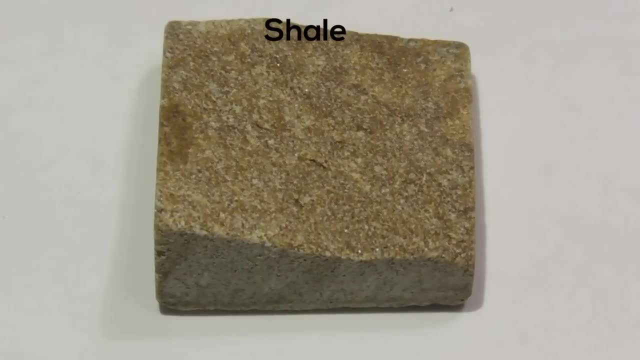 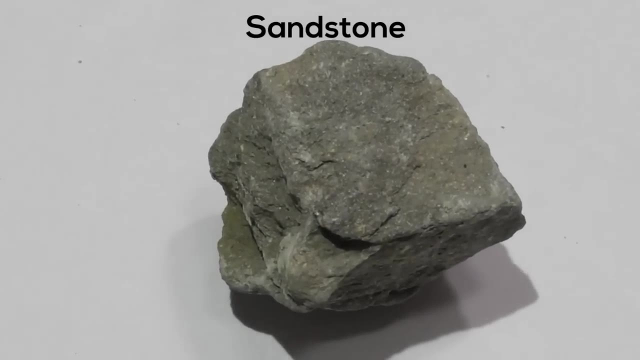 especially quartz and calcite. Shell is very fine-grain. Next, Sandstone. Sandstone is one of the most common types of sedimentary rock found across the world. They are clastic sedimentary rocks. all in all, They are made up of the black silt size Victoria. 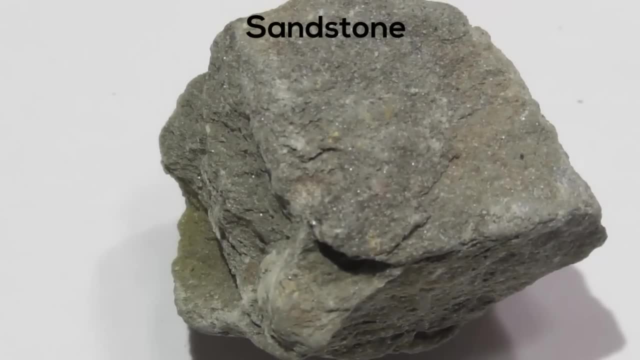 the sauce of the great scissor and sea pot of rock, All the rock that grows without odour As they form theandi 서라, and flora are discovered around them. These rocks are also called sedimentary rocks, rock composed of sand sized grains of mineral rock or even organic material. 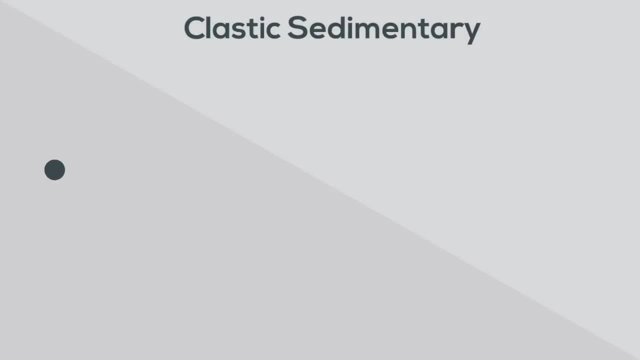 Clastic sedimentary rocks are subdividing according to the dominant particle size. These particle sizes are ranked from smallest to largest. Clay is the smallest, then silt, sand, gravel, pebble and boulder Up first Shell. Shell is a fine-grained clastic sedimentary rock composed of mud. 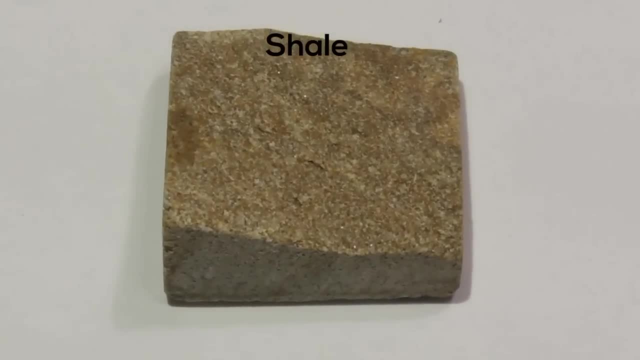 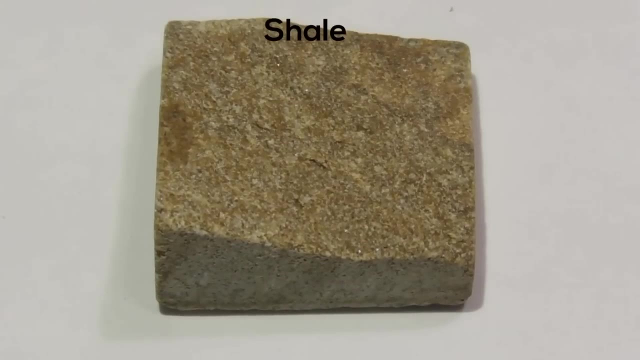 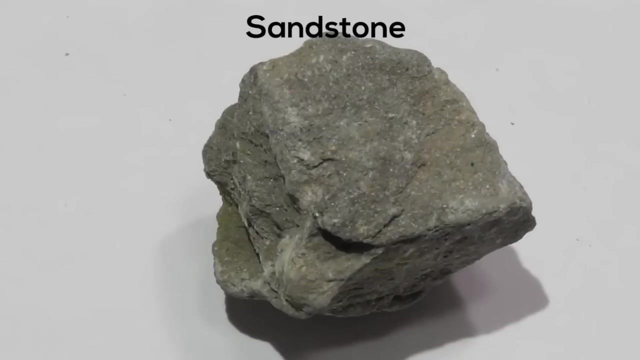 This mud is a mix of flakes of clay, minerals and silt-sized particles of other minerals, especially quartz and calcite. Shell is very fine-grained. Next, let's look at Sandstone. Sandstone is one of the most common types of sedimentary rock found throughout the world. 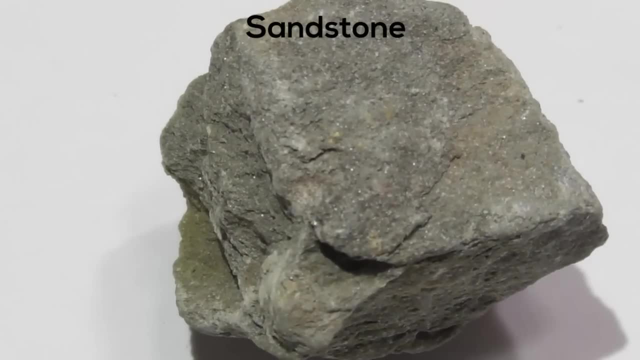 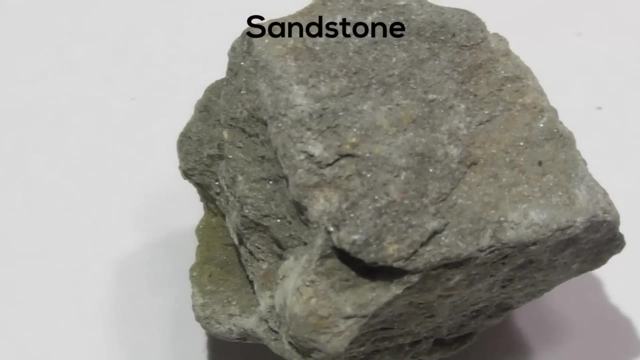 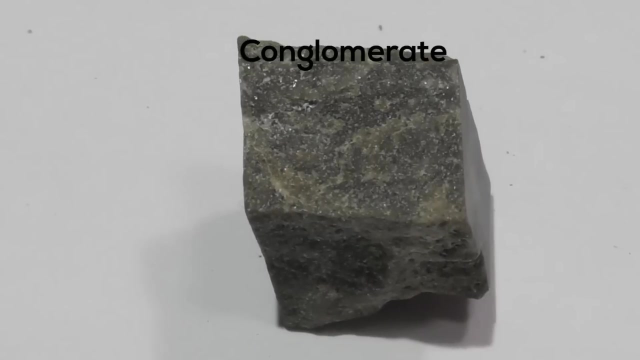 It is a clastic sedimentary rock composed of sand sized grains of mineral rock or even organic material. It also contains some cementum, material that binds the sand grains together. Next, Conglomerate Conglomerate is a coarse-grained clastic sedimentary rock composed of pebbles and boulders. 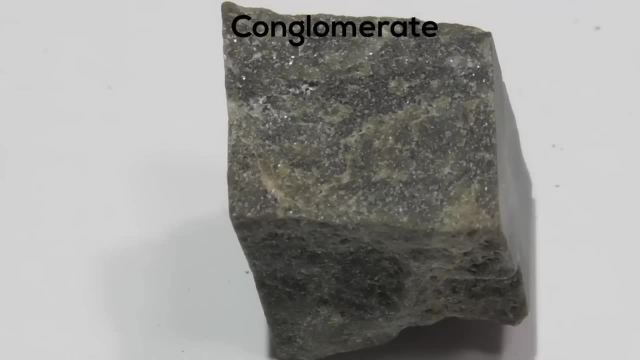 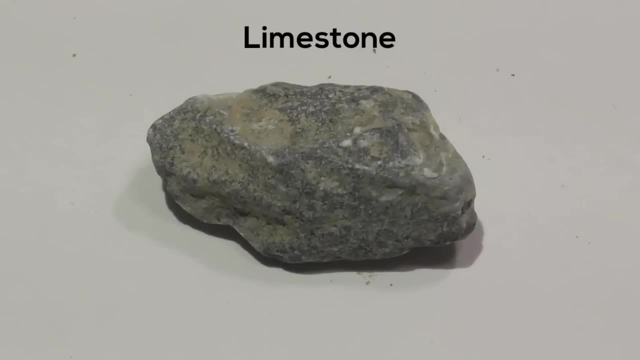 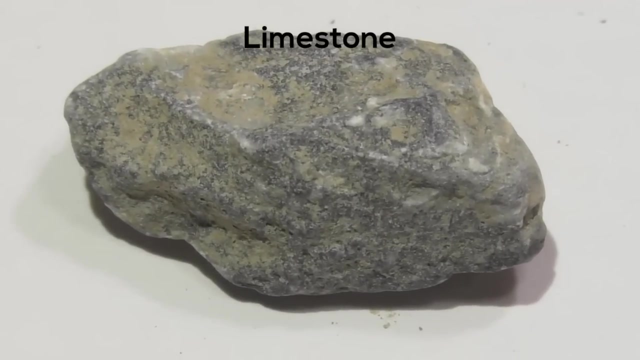 Between these pebbles and boulders is generally filled with smaller particles of calcite or quartz cement that binds the rock together. And finally, limestone. Limestone is an organic sedimentary rock that is often composed of the skeleton fragments of marine organisms such as coral. 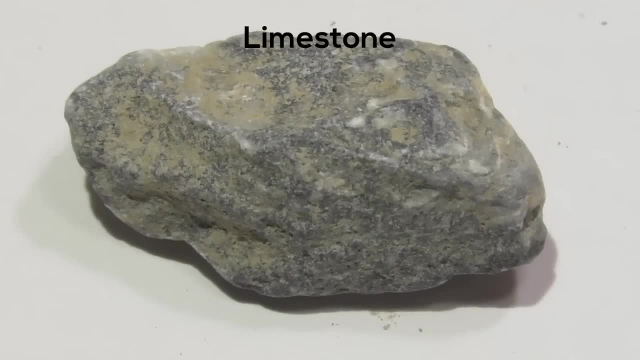 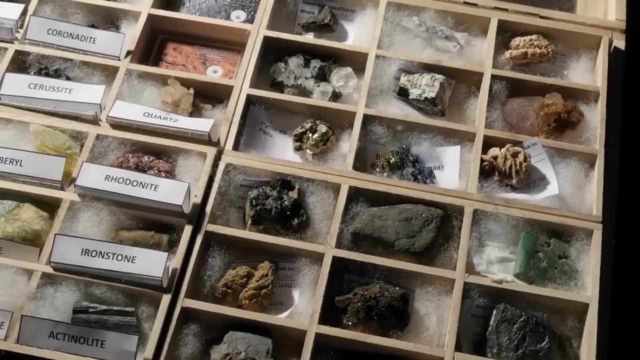 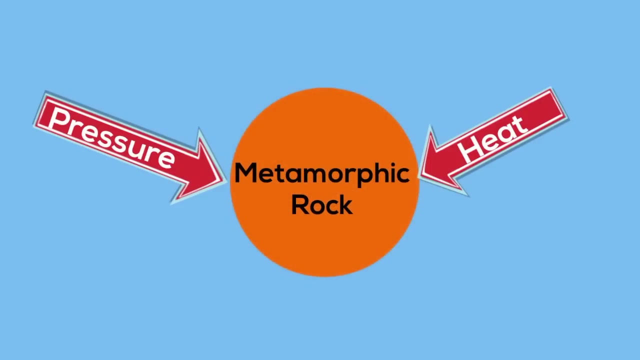 About 10% of sedimentary rocks found on earth are limestones. Metamorphic rocks come from existing rocks that are subjected to extreme heat and pressure. This heat and pressure changes the original structure into a new type of rock. Sedimentary, igneous and even metamorphic rocks can all become metamorphic rocks when 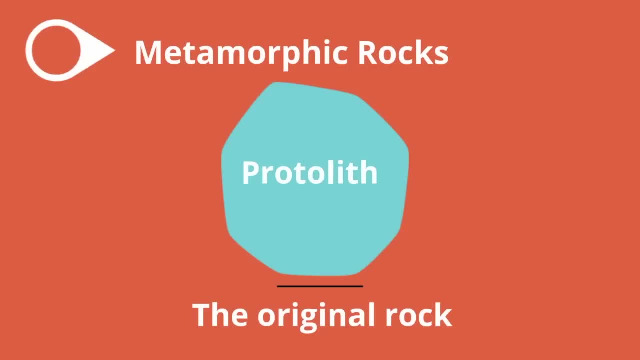 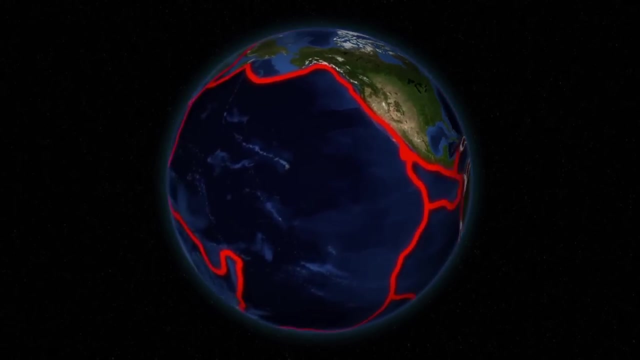 exposed to heat and pressure. The original rock is the protolith, but is commonly referred to as the parent rock. Metamorphic rocks can form deep in the earth's crust Or at areas of plate tectonic movement. Two major types of metamorphic rocks are foliated rocks, which have crystals in stripes and non. 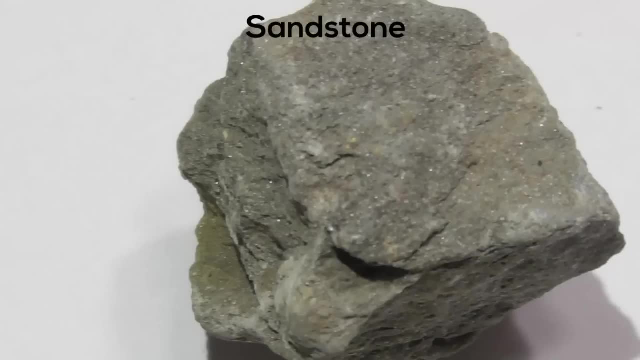 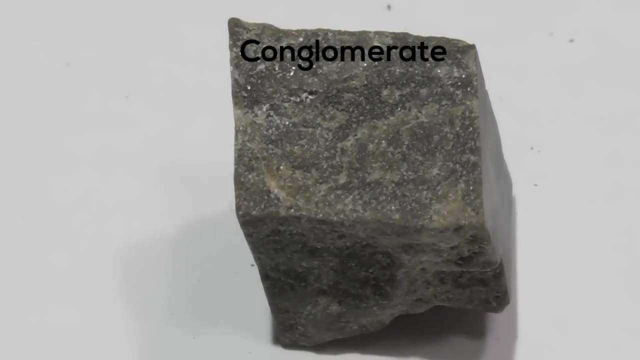 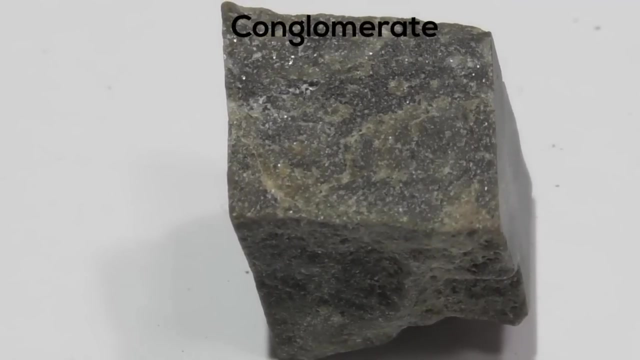 It also contains some cementum, material that binds the sand grains together. Next, conglomerate: Conglomerate is a coarse grained clastic sedimentary rock composed of pebbles and boulders. The space between these pebbles and boulders is generally filled with smaller particles. 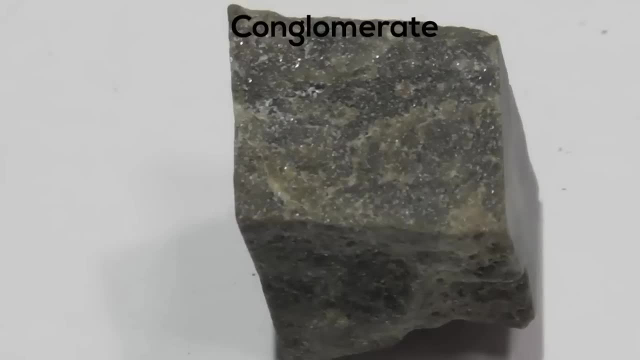 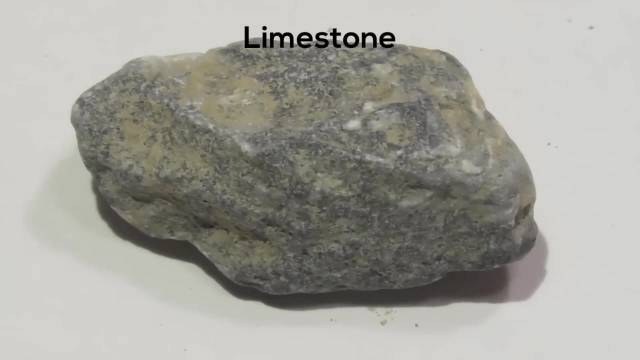 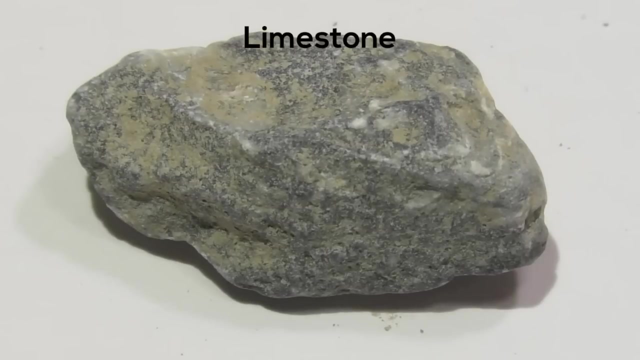 of calcite or quartz, cement that binds the rock together. And finally, limestone. Limestone is an organic sedimentary rock that is often composed of the skeleton fragments of marine organisms such as coral. About 10% of sedimentary rocks found on earth are limestones. 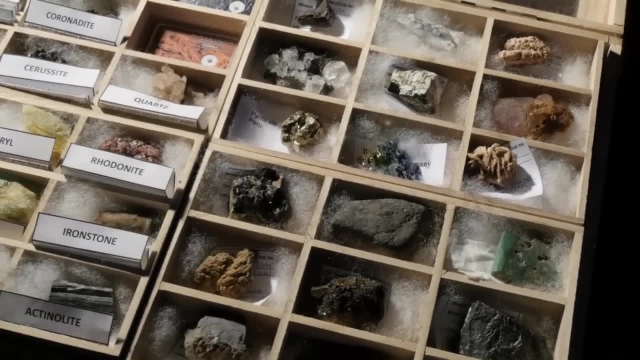 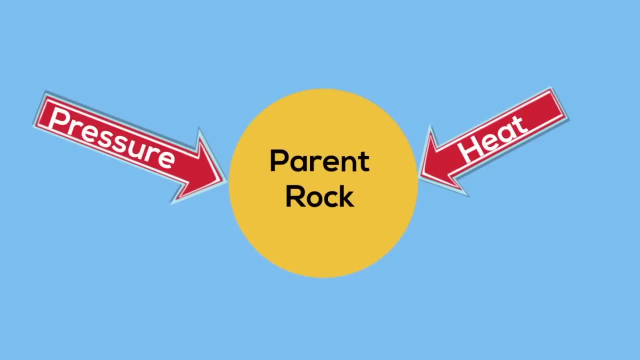 Metamorphic rocks come from existing rocks that are subjected to extreme heat and pressure. This heat and pressure changes the original structure of the rock. The rock is then transformed into a new type of rock. Sedimentary, igneous and even metamorphic rocks can all become metamorphic rocks when 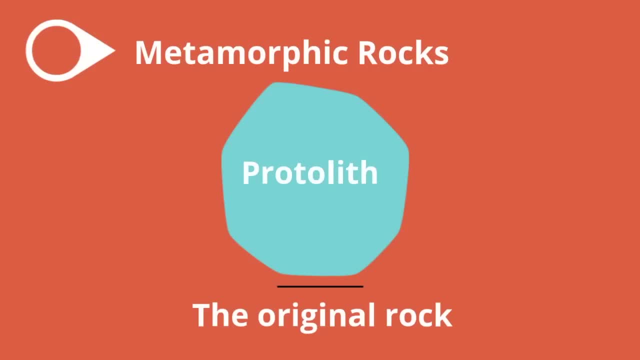 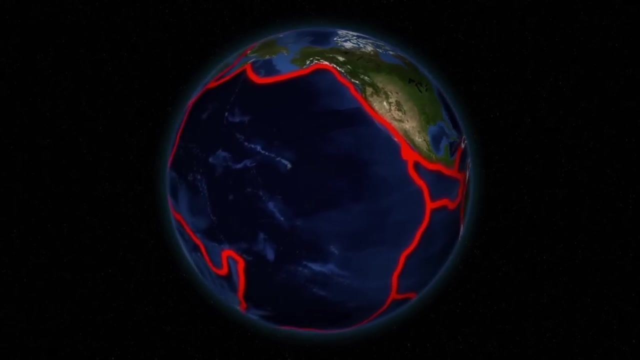 exposed to heat and pressure. The original rock is the protolith, but is commonly referred to as the parent rock. Metamorphic rocks can form deep in the earth's crust or at areas of plate tectonic movement. Two major types of metamorphic rocks are foliated rocks. 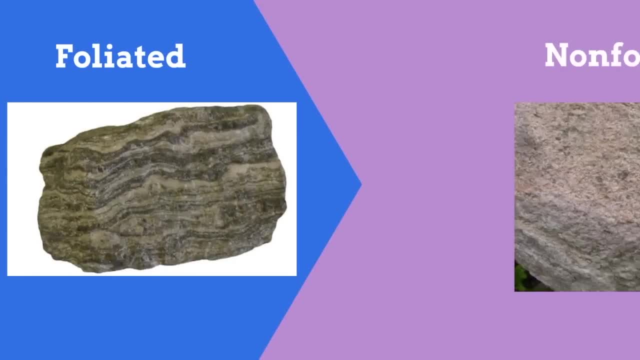 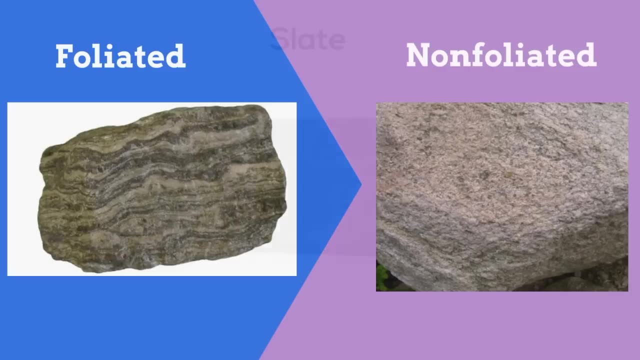 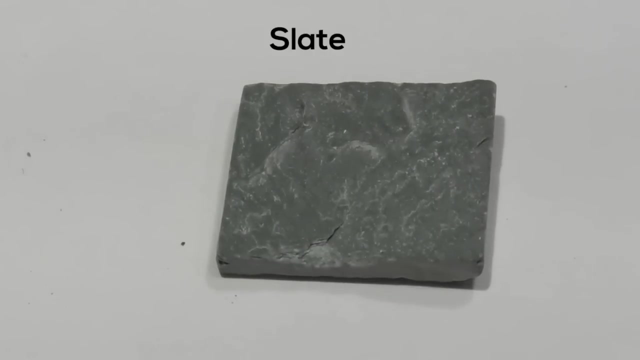 Foliated rocks- They have crystals in stripes- and non-foliated, which do not have crystals in stripes. So let's take a look at some common metamorphic rocks. Slate has very, very small minerals. It is considered foliated and its parent rock is shale. 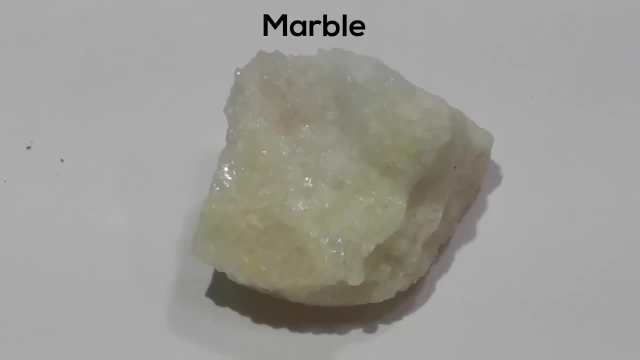 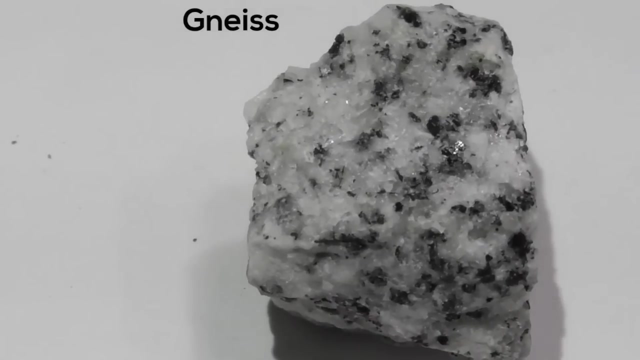 Marble has fine to medium crystals. Its parent rock is limestone and it is considered non-foliated. Quartzite is a non-foliated metamorphic rock and its parent rock is sandstone. Gneiss is a foliated rock and its parent rock is schist. 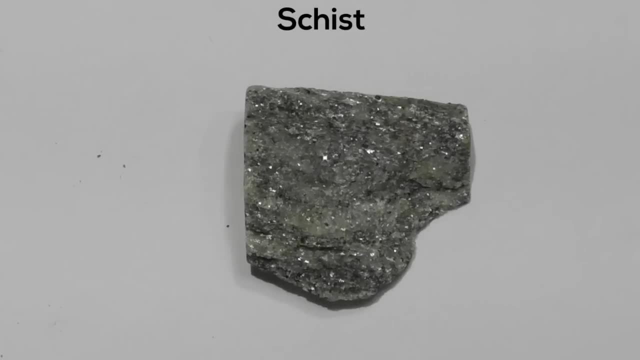 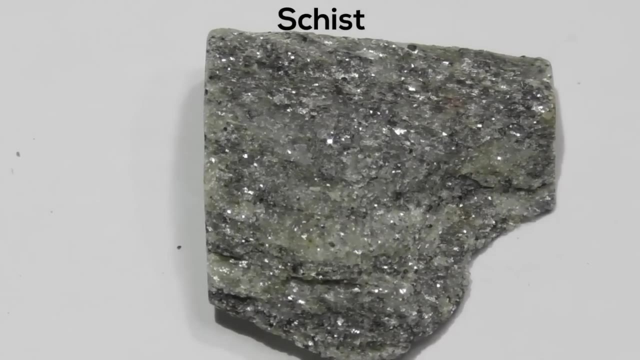 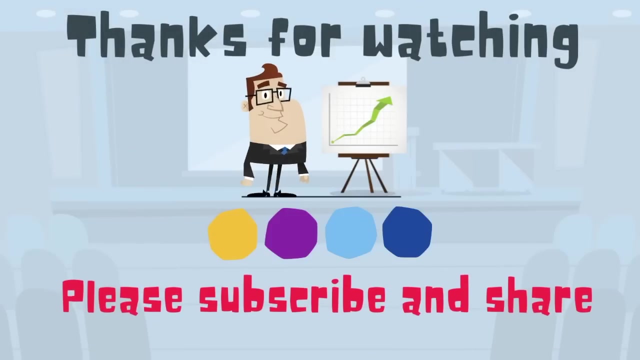 And finally, Schist is a foliated metamorphic rock and its parent rock is slate. If you need to know more about metamorphic rocks, This playlist should help And, as always, thanks for watching, and MooMooMath uploads a new math and science video every. day. Please subscribe and share.